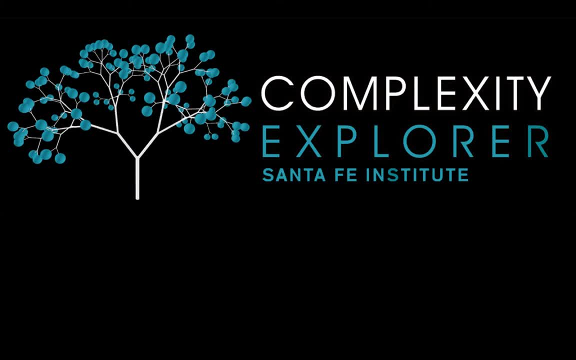 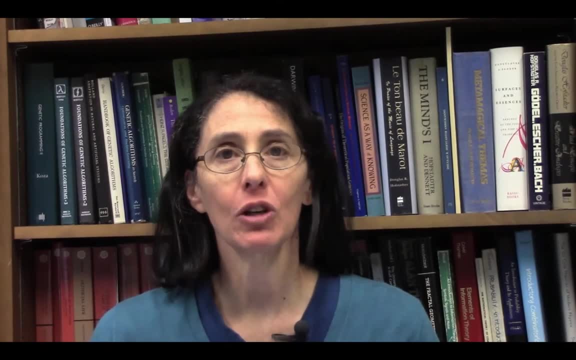 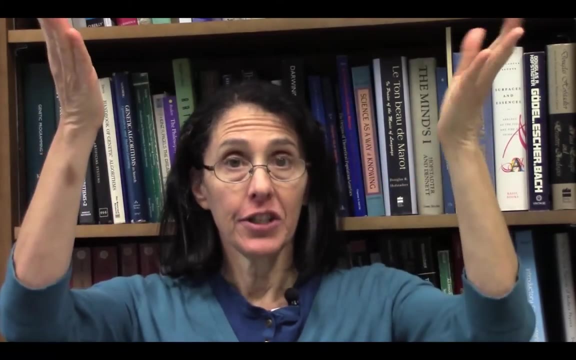 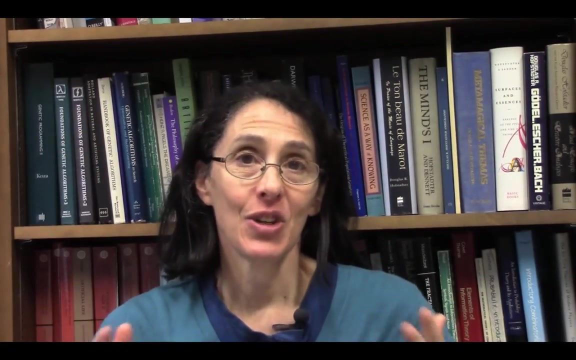 Hello everybody. This unit is on fractals. Fractals are objects that are self-similar at different scales. Think of a tree: It has a trunk that has branches, and those branches themselves have branches coming off of them, and those have sub-branches, and so on. So 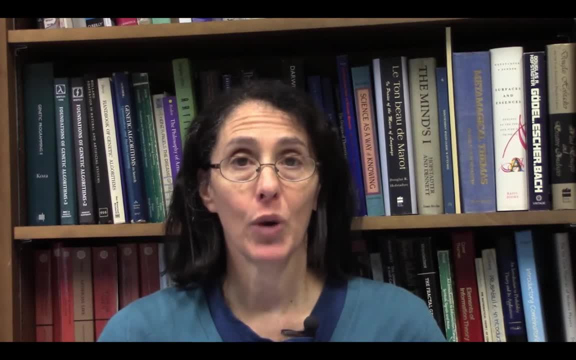 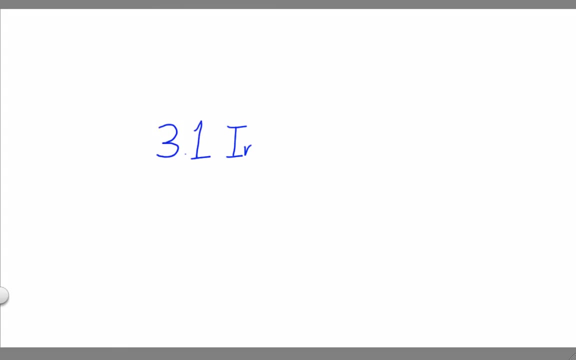 that's a fractal. Fractals turn out to be a good way to describe many objects in nature. In this unit, we'll explore fractals both visually and mathematically, and I'll survey some of the roles played by fractal geometry in complex systems. 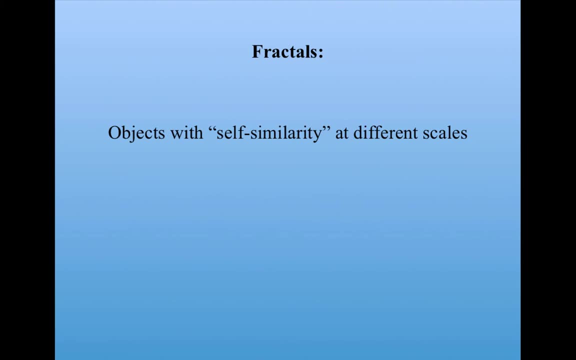 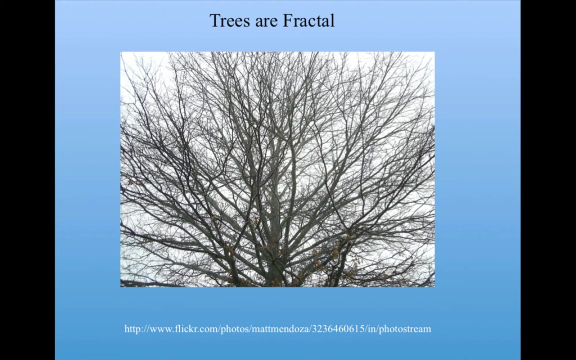 Fractals can be intuitively defined as objects with self-similarity at different scales. It's striking how many natural objects there are with this group. Let's look at a simple example: Trees. Trees are fractal, and let me explain the notion. 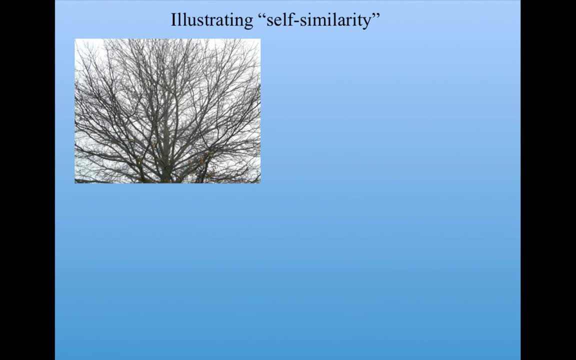 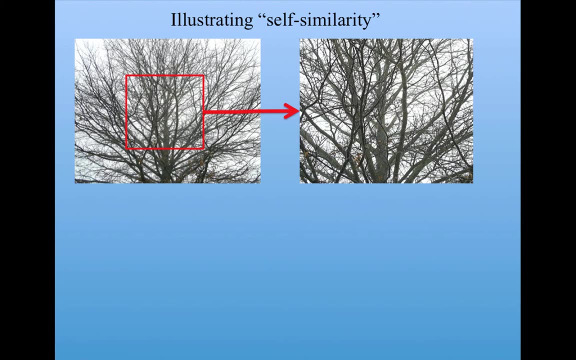 of self-similarity. Let's take a picture of a tree. Now we'll take part of that picture and crop it out and blow it up. You can see that the structure of this blown-up part of the picture is very similar to the structure of the whole picture itself. Well, let's do. 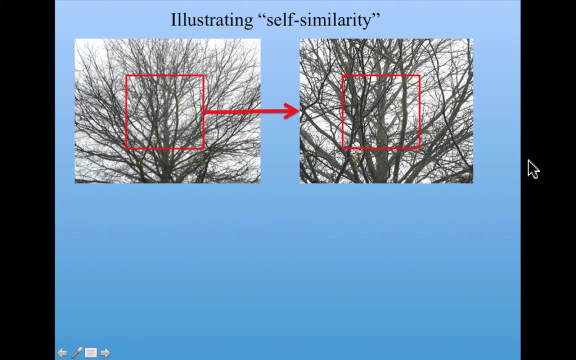 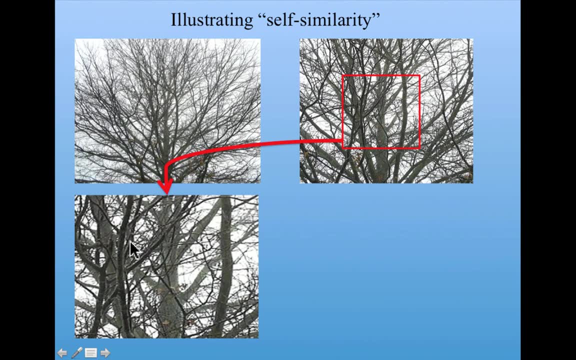 that again. Let's take a part of this picture within this red box and let's blow it up Again. the structure that you see inside this blown-up part of this picture looks very similar to the previous two pictures, And notice that this third picture is a very tiny part of. 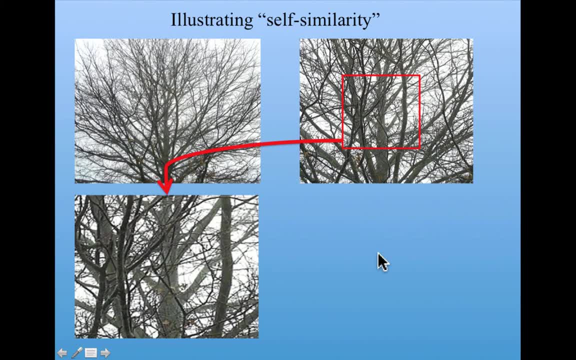 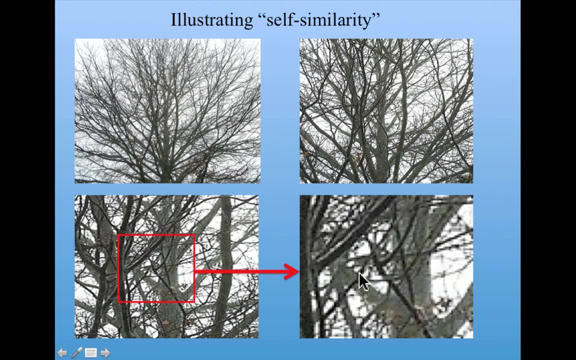 this original picture. Now we can do that same thing again. Take a part of this third picture. blow it up Again. we have structures that look very tree-like. So no matter how far down you go, up to a certain point in these pictures, you can keep taking little crops, blowing them up and seeing. 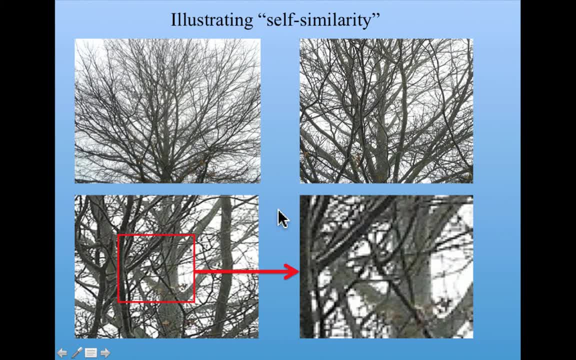 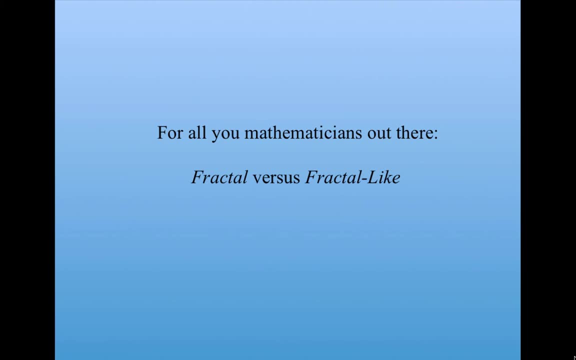 that they have very similar kinds of structure. That's the crux of the notion of self-similarity at different scales. Now, before I go further, let me make a quick note for all of you mathematicians out there. The actual definition of fractal means that the object is perfectly self-similar at all. 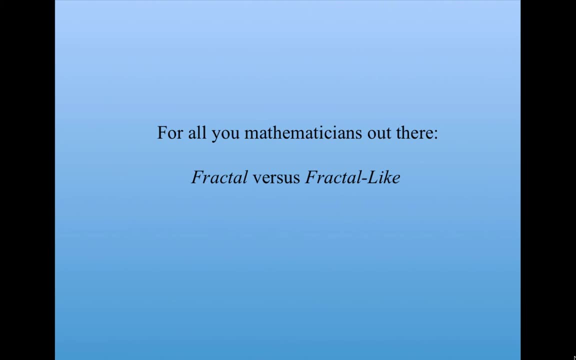 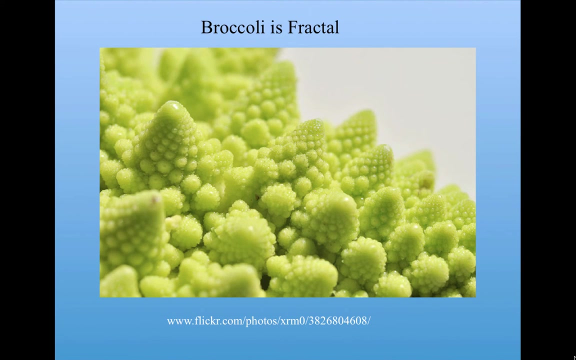 possible scales. So the objects that we're going to talk about in nature are only fractal-like. They're not real fractals from the mathematical sense, But I'm going to use the term fractal to describe them anyway. So here's a picture of a special kind of broccoli that has fractal properties. You can. 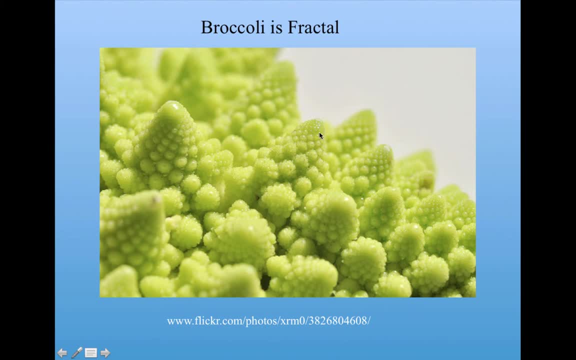 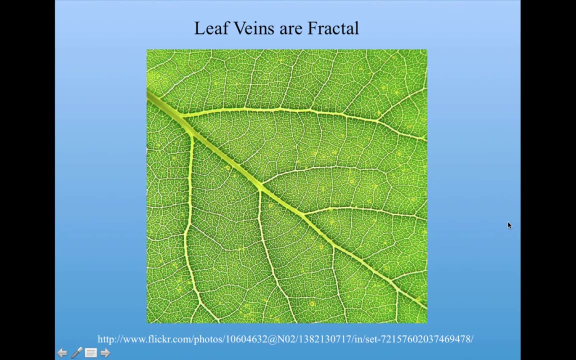 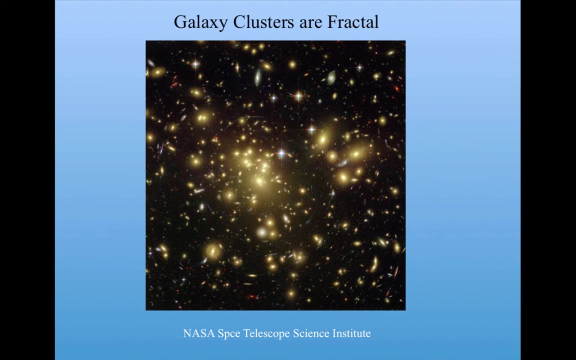 see that each of these little broccoli mounds consists of other little mounds that themselves have the same structure, and so on. Leaf veins are fractal, in the same way that trees are fractal. Galaxy clusters can be fractal. This is actually a cluster of clusters, and if I looked at one of those clusters, that itself would be a cluster of clusters. If I had one of those clusters, that itself would be a cluster of clusters. This is how fractal works. In the same way that we concentrate eyeshadow to psi, we put a cluster of glasses on each other, past and next to each other, called upper and lower. 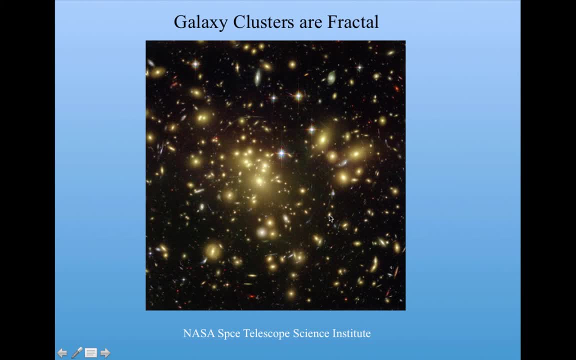 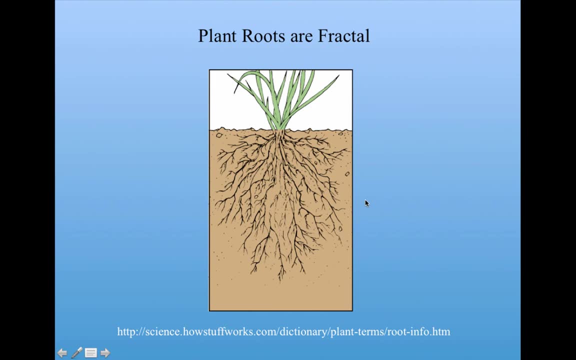 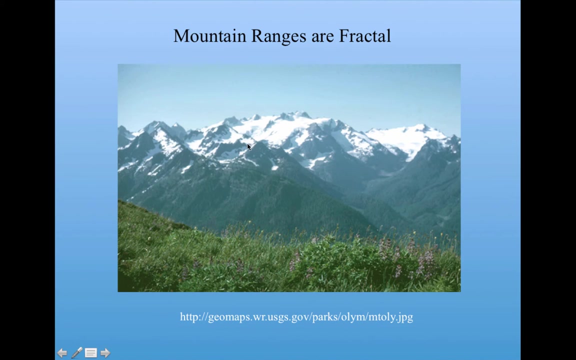 and so on. So galaxy clusters can be fractal. Plant roots have tree-like fractal properties. Mountain ranges are fractal. If I look at any one of these mountains, it also has peaks and valleys, the same way that the whole mountain range. 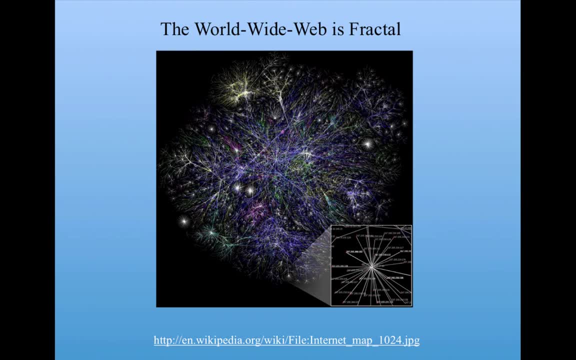 does. Surprisingly, the World Wide Web is a fractal. This is a map of part of the World Wide Web, the connections between web pages, And you can see. if you blow up a tiny part of it, it has the same kind of spike. 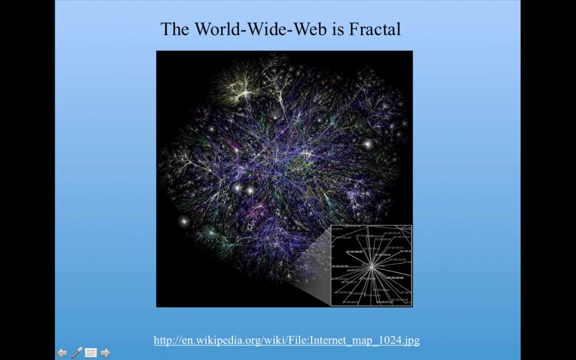 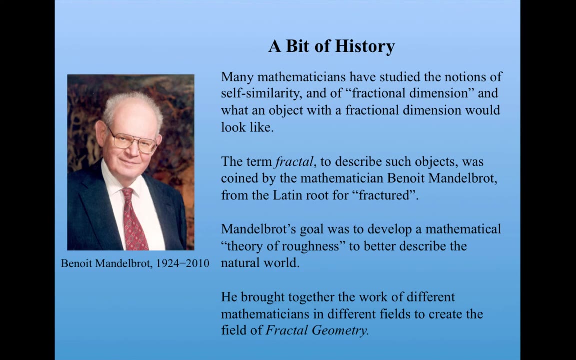 coming out of a central hub that the whole web picture does. So we'll see later, when we talk about networks, the significance of the fractal properties of networks like the World Wide Web. Those are a small sample of some fractal-like objects in nature. 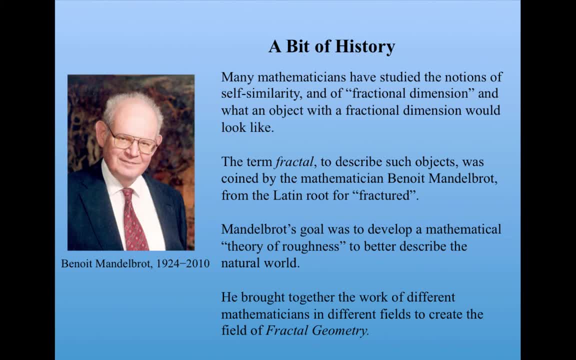 To talk about a little bit of history. many mathematicians studied notions related to fractals, such as the notion of self-similarity or fractional dimension- And we'll talk about that also a little bit later on- And it looked like what objects with fractional dimension would be like. So that's going back many. 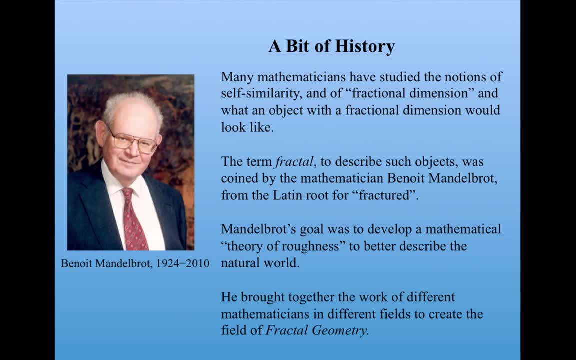 centuries in mathematics, But the term fractal itself to describe such objects was coined by Benoit Mandelbrot, a 20th century mathematician. He took the name from the Latin root for fractured Now. Mandelbrot's goal was to develop a mathematical theory of roughness. 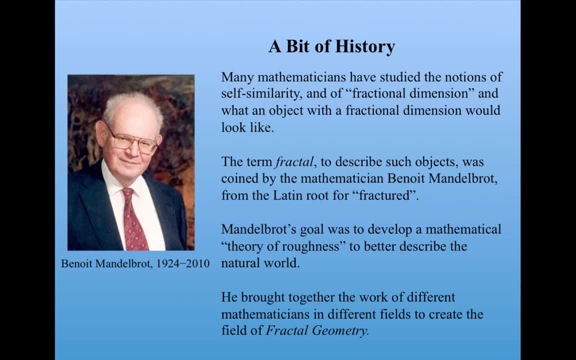 to better describe the natural world. Typical geometry, the mathematics of simple structures, describes smooth objects, But the real world actually consists of very rough objects like mountain ranges and galaxy clusters and so on, And Mandelbrot realized that he needed to bring together 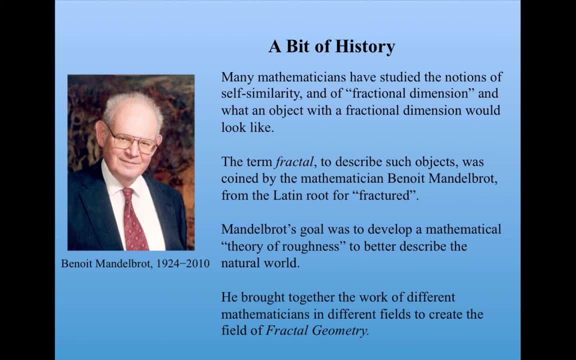 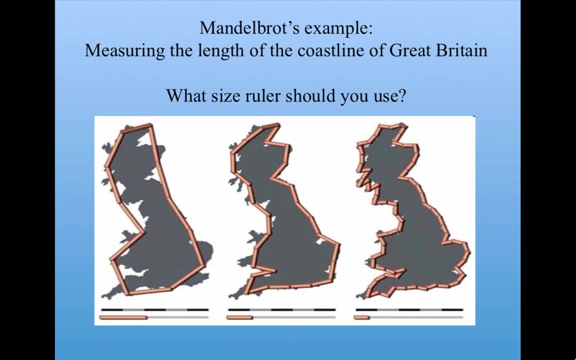 the work of many different mathematicians in different fields to create a new sub-branch of mathematics called fractal geometry. Mandelbrot's most famous example is the notion of measuring the length of a coastline. He particularly looked at the coastline of Great Britain because of 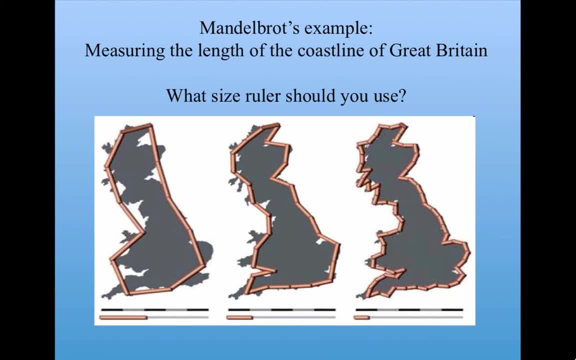 its ruggedness. And his question was: suppose we want to measure its length. What size ruler should we use? Well, if we look over here, we're measuring it with a rather long ruler And we get a certain number of lengths. 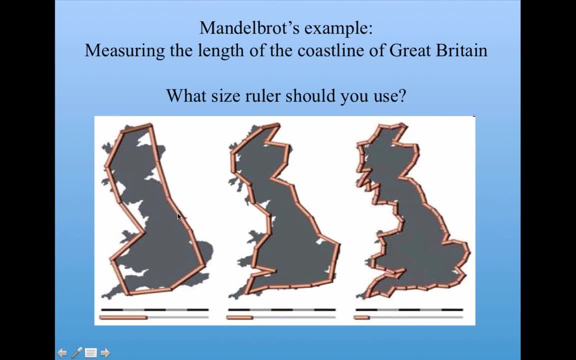 1,, 2,, 3,, 4,, 5,, 6,, 7,, 8,, 9,, 10,, 11,, 12.. But if we shrink the ruler we actually get a longer coastline. Here we shrink it by half and if you count them up, 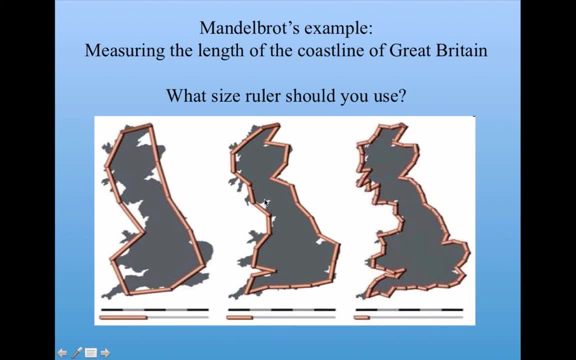 you get 1,, 2,, 3,, 4,, 5,, 6,, 7,, 8,, 9,, 10,, 11,, 12,, 13,, 14,, 15,, 16,, 17,, 18,, 19,. 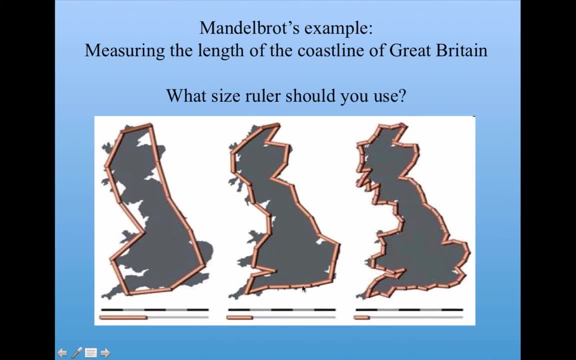 20,, 21,, 22,, 23,, 24,, 25,, 26,, 27,, 28,, 29,, 30. And 28 is more than 2 times 12.. So that means that the actual length we get 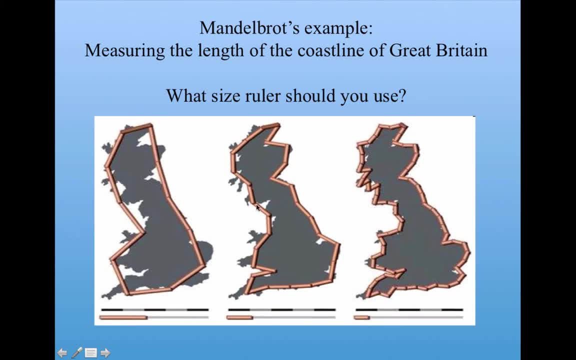 here is longer than the length we get here, And the reason for that is these smaller rulers can fit a little bit better into the nooks and crannies that we see on the coastline. If we look at an even smaller ruler, we cut this one in. 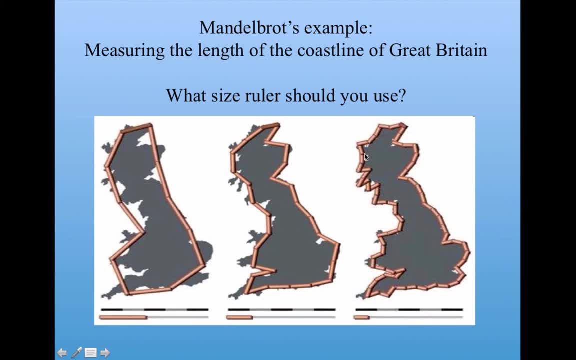 half, you can see that it fits even better into more nooks and crannies. Okay, And we'll give us a longer coastline than we measured here. So what is the real length of the coastline? If we looked at an even smaller ruler, we'd obviously be. 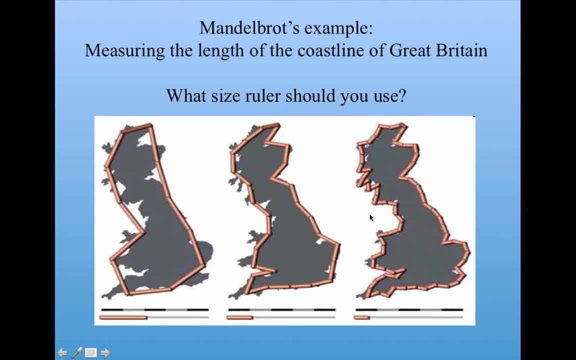 able to fit into all these little other nooks and crannies. And the nooks and crannies, as you know, go very far down as we zoom in on the coastline. Let's see a version of this with real coastline pictures. Here I chose the coastline of. 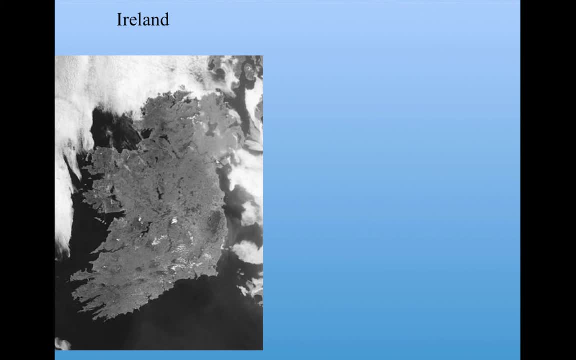 Ireland. Here's a satellite picture of Ireland. So let's play the same game here that we did with our tree before We take a small bit of the coastline. We see that it's, you know, fairly. this is a fairly rugged coastline, especially over. 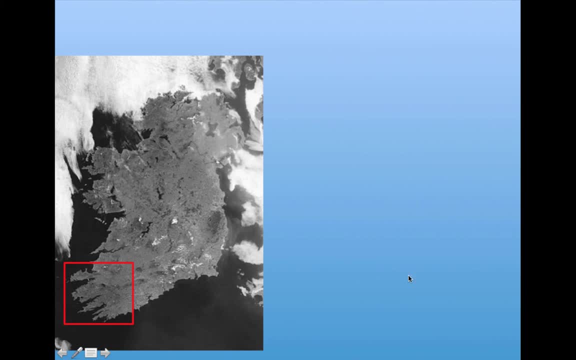 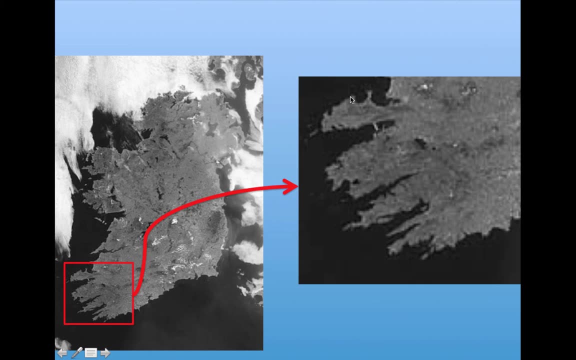 here in the southwest part of Ireland. So what I'm going to do is now blow this up, And now we can see even more nooks and crannies, So we can imagine sticking a smaller ruler into here and getting a longer measurement for the coastline. 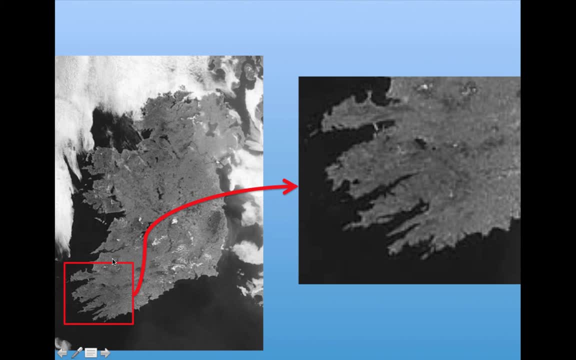 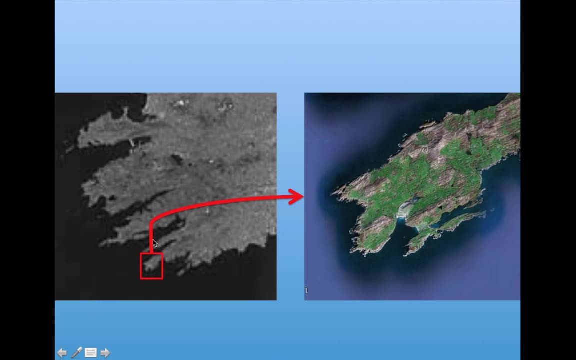 than if we measured it at this scale. Now I can do the same thing: Take a little bit of this and blow it up. I do that on the next page, where I blow up this bit. Now I moved from using a satellite picture to a Google Maps picture, And now I can see even more little tiny nooks. 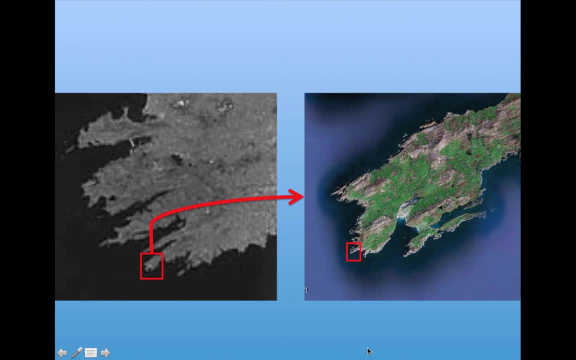 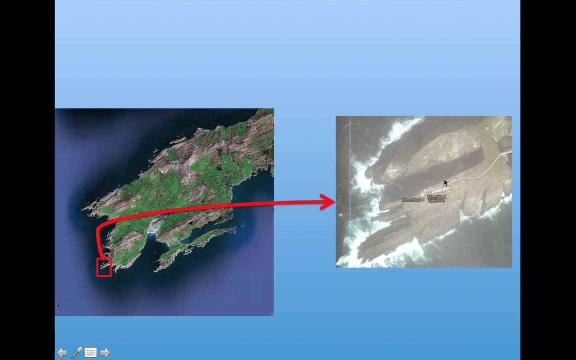 and crannies in the coastline. Do that to this little bit over here. Now, remember, that's not the same as this little bit over here. It's a little tiny bit of that little bit. Take that little bit, blow it up. You can't see it as well now, but you can see. 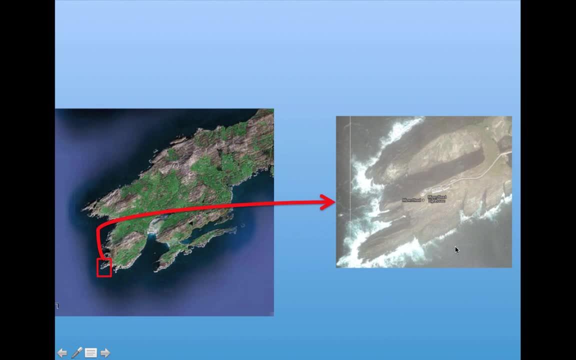 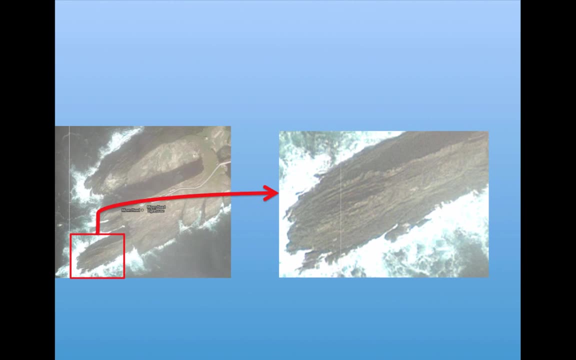 now even more detail down here, Even more roughness at a smaller scale. Now we can keep doing this over and over again. Here's this part blown up. We see more detail, And if we blew up a little part of this, Google Maps actually doesn't go.